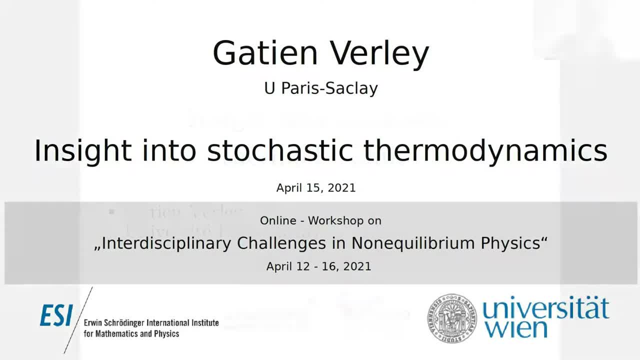 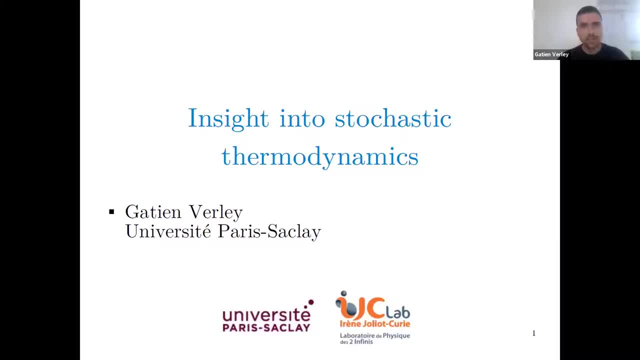 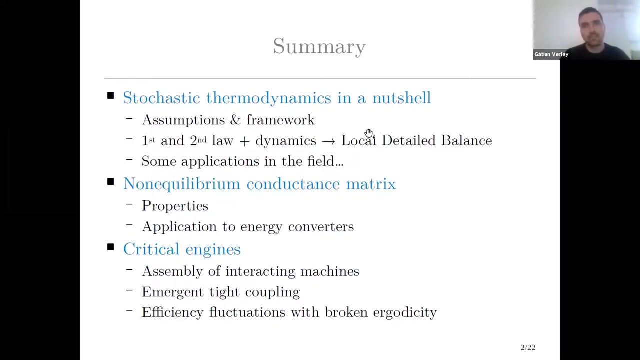 So I continue on the physics of small thermodynamic systems and I want to give a kind of introduction talk to stochastic thermodynamics first, basically justifying the local detail balance Jan-Maria just told us about in the various systems that can be out of equilibrium in the various ways said. 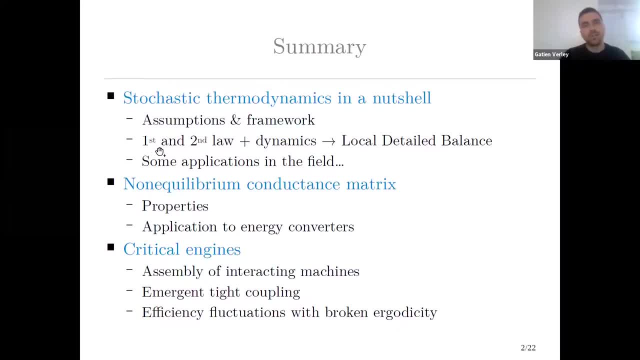 And this comes from the compatibility of two definitions of entropy productions, one from the dynamics and one from physical observables that appear in the second law and first law. So basically, heat is defined by looking at the first law. it also appears in the second. 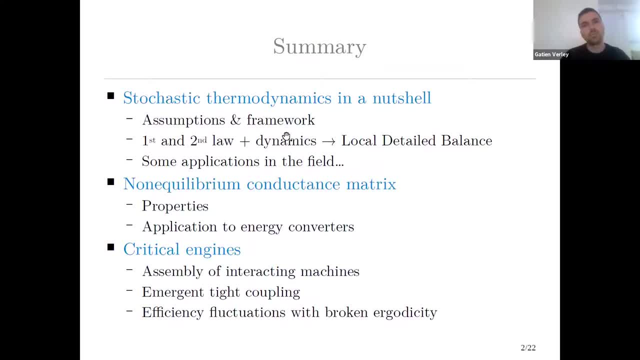 law And due to the fact that you have a dynamical definition of entropy production, you must relate dynamics to physics through the heat definition. So this is local detail balance and basically this is why the theory is so general, because you don't need so much assumption. You 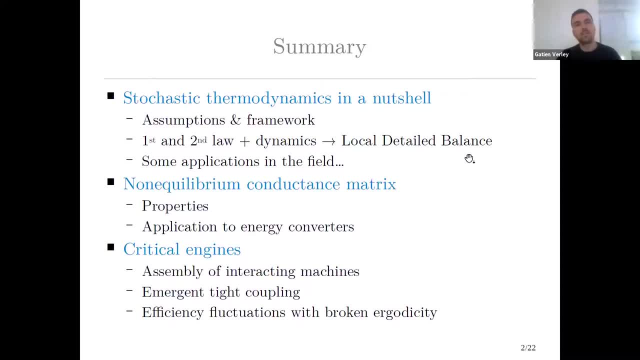 should have a thermodynamic consistency in the theory, and this is what is about stochastic thermodynamics. And then you have many applications of that that I will try to. I mean, I will give a quick overview of it. Then I move to my own work, more precisely to the work of my collaborators, and I mean myself and my team. 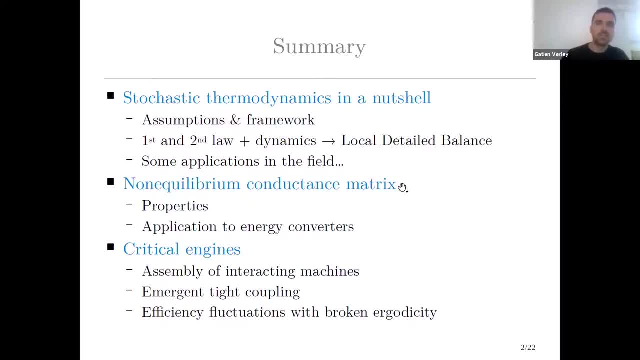 The first topic is non-equilibrium conductance, which is a generalization of Onsager response matrix to the nonlinear case, And I give application to energy conversion. and then I continue with the topic of energy conversion with critical engines, because it has helped. 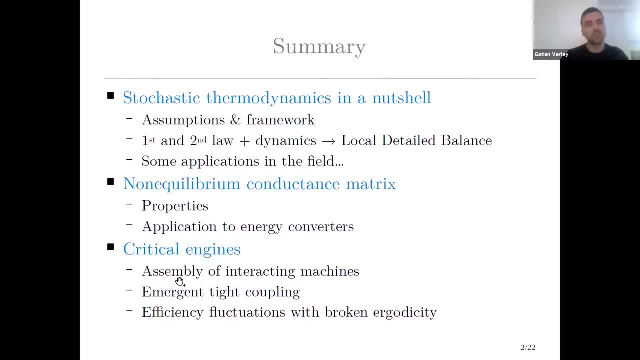 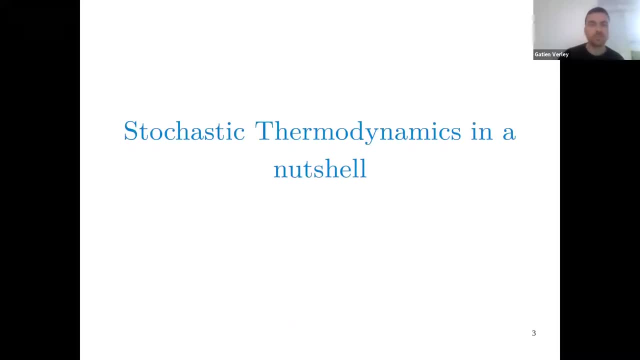 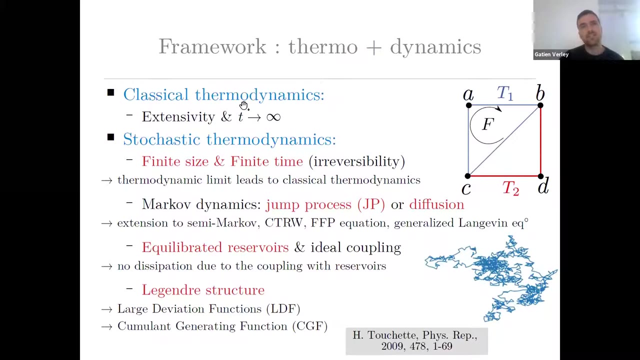 us to understand the physics that is going on. And then I continue with the topic of energy conversion with critical engines, because it has helped us to understand the physics that is going on. So first the stochastic thermodynamics: overview: Classical thermodynamics: use, extensivity, large size systems and reversibility or a long time. 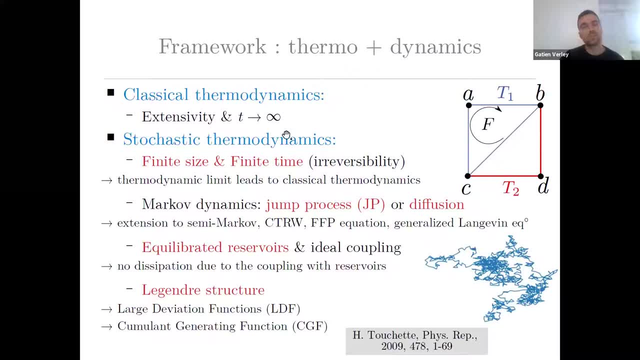 limit And in the cycle you always have reversible steps so that you can reach equilibrium. states and states function differences between those states. On the opposite, stochastic thermodynamics deals with finite size systems and that are evolving in finite time, or in stationary states that are irreversible. You may take Markov dynamics either jump processes on the graph. 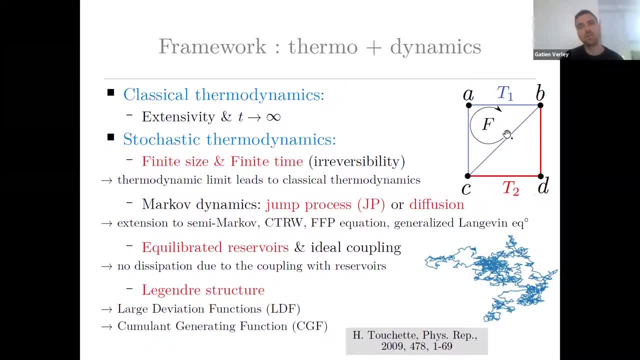 between different states or diffusive processes, or even a mixture of the two, like a molecule that is diffusing and changing of conformation. But this is mainly not a requirement. You have extensions to, for instance, semi-Markov processes or the related topic of continuous 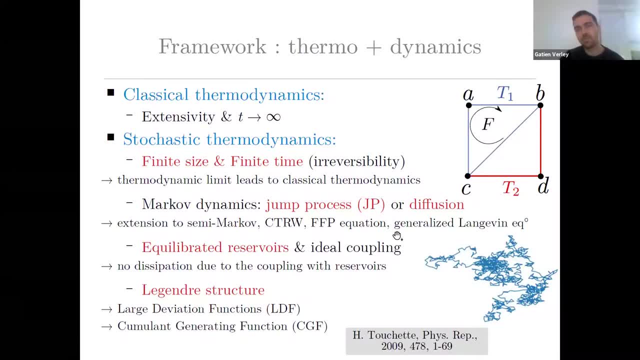 time random walks. You have OTAs made work on generalized normal equations where the drag force is produced by a kernel. What is required is an ideal coupling to the reservoir that must remain at equilibrium. So this is a strong assumption. Reservoir must be. 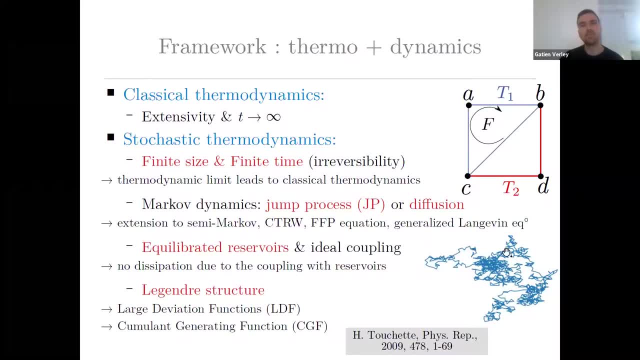 very big and then they are not disturbed by the system even though it is far away from equilibrium. And in stochastic thermodynamics we used to study the probabilities and we use large deviation theory for that, where we have a Legendre structure between the large deviation function. 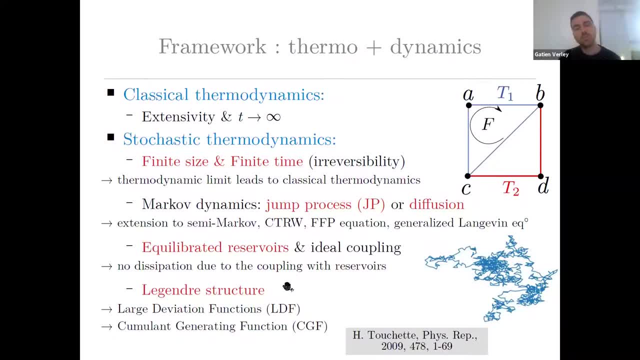 which is basically the log ratio, the log of a probability distribution after a long time. So it's an asymptotic evaluation of a probability distribution and the communal generating function, which is related by Legendre transform, And this is well explained in the report of. 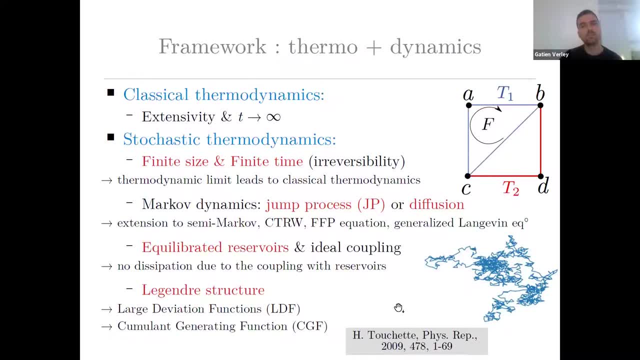 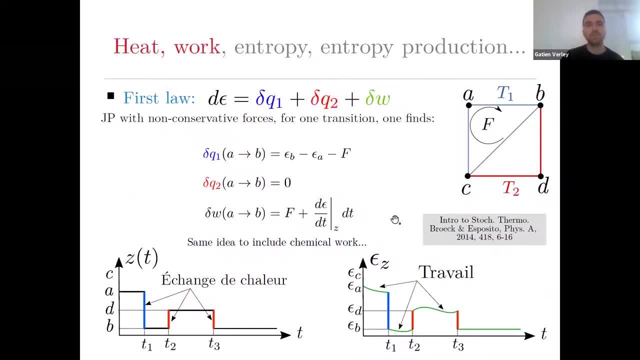 Tuchel, this large deviation theory applied to statistical physics, which is basically a large deviation theory. Okay, so let's go to our main message about stochastic thermodynamics, which is that the agreement between the first law and second law in the definition of heat. 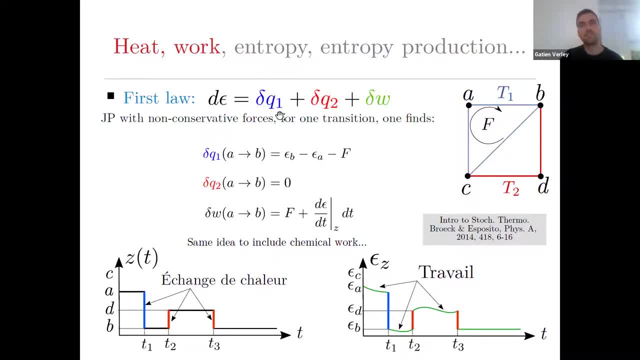 lead to a dynamic constraint, So I must have terminic consistency. So let's look at the first law over an infinitesimal times step, and this change of energy with be related to heat absorbed from a cold reservoir, heat absorb from a hot reservoir and also the work received. by the system. S after before first amchemistry, Anh after energy. Ch is node Sam. GR are the reinforcements of the initial constant, So they are a coincident between the tua and the d by the sin. This is happen when a rich油 component of state. 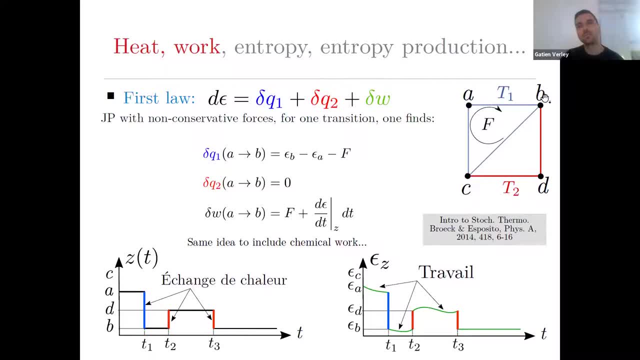 And this change of energy will be related to heat absorbed from a cold reservoir, heat absorbed fire and heat absorbed from a hot reservoir, And also the work received by. So, for a transition, during this small time step from A to B, I will have a heat exchange, which is the energy difference between the two states and eventually decreed by the work received by the system. 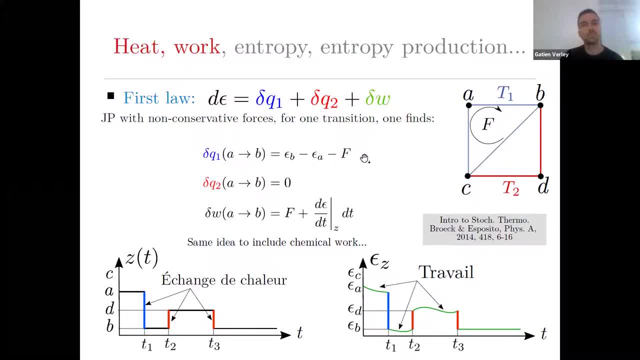 Here I take the force equal to work, because displacement is one, for instance, And I say that during this transition, heat is just coming from the reservoir one, not from the reservoir two, because this is the reservoir that triggers the transition, that keeps the energy. 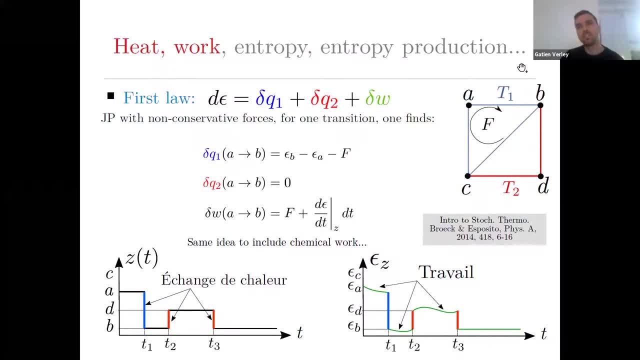 And I could have drawn another hedges here in red so that I would have another transition and then it would be another description here. But for this edge here I have no heat, I have no heat exchange with the hot reservoir And I have work that has been done, which is this F I was speaking about- removed from the heat, plus, eventually, a contribution that is due to the evolution in time of my energy levels. 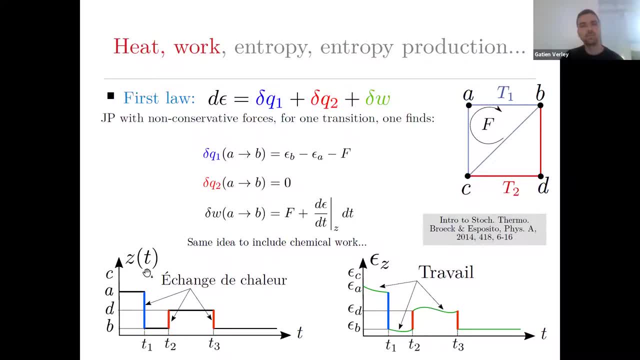 The system is going through different. Can I move this? Yes, I can. That is undergoing some transition at various times And the heat is just The change of the energy during the transition and the work is the change of the energy away from the transition. 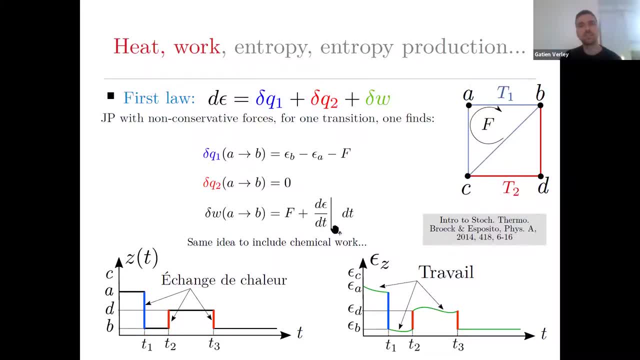 And this is this contribution at given states, which is the state of the system at time t. But you can include many other things in the work and in the heat through, for instance, like chemical work, And you just add it and remove it. 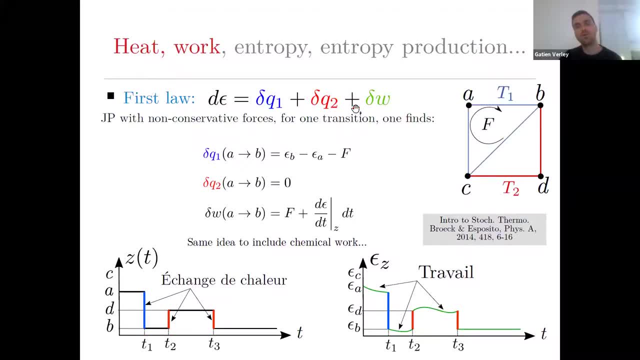 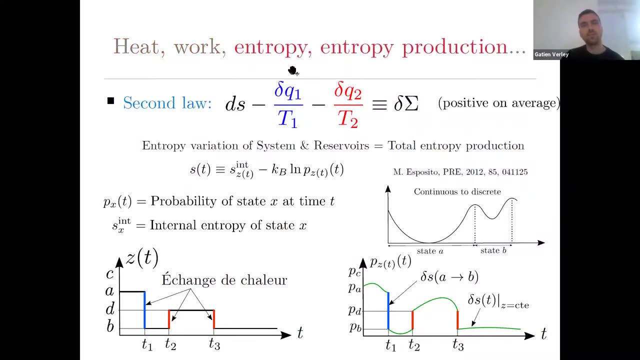 And the rest is just the first theorem of analysis, I mean mathematics, just Okay, It's just two way of varying a quantity: through the state or through the time. This is the first law. The second law, at the macroscales, tells us that the change of the system entropy and the change of the reservoir's entropy should give you your entropy production. 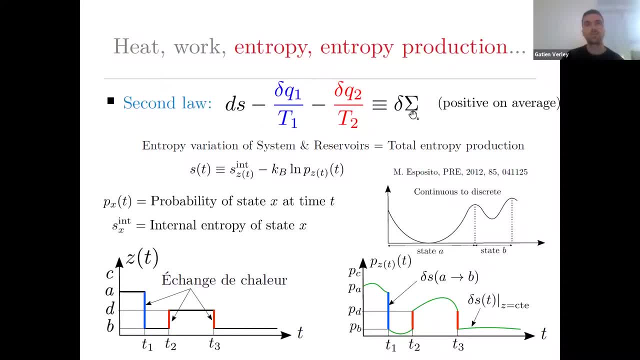 So if you have good definition for everything, you should have a constraint on your dynamics if this definition involves your dynamics. The definition of the entropy was given by Jan Maria, I think, and he emphasized the internal degrees of freedom a little bit in the end of his talk. 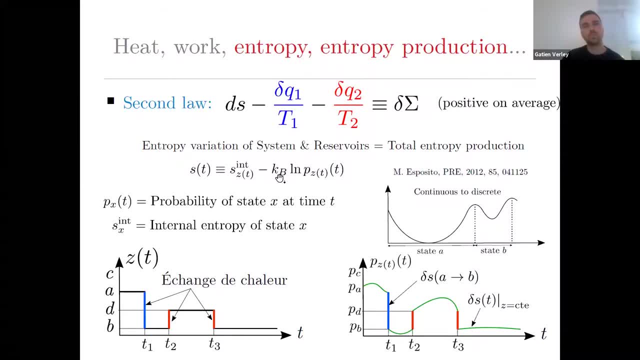 So there is a contribution which is a Shannon contribution- On average, this would give the Shannon entropy- And there is an internal entropy which is related to the fact that you may have a more precise description of your model. So you must have this freedom in the internal states. 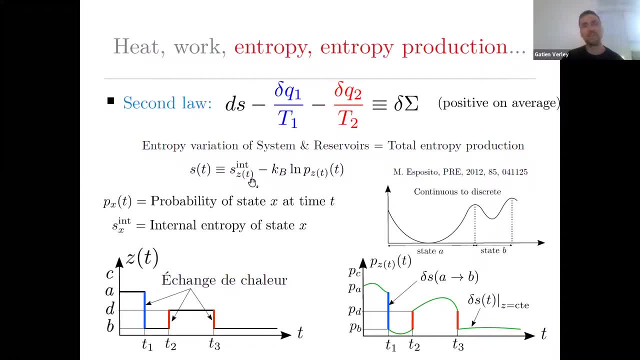 So that the theory is consistent across change of scale. And then if you have this second law with, Okay Here this is a stochastic quantity because the probability is evaluated at a stochastic state. If you have this second law, that is true for your physical observable. 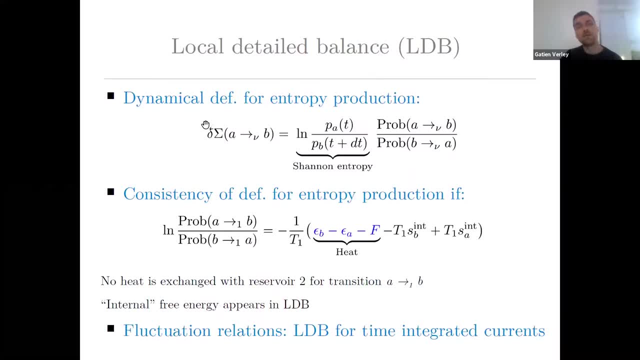 But that is also true for the dynamics. Okay, If you have this second law, that is true for your physical observable, But that is also true for the dynamics Given by the following statements: that the entropy production during the jump is just a log ratio of the probability in one direction and the other direction. 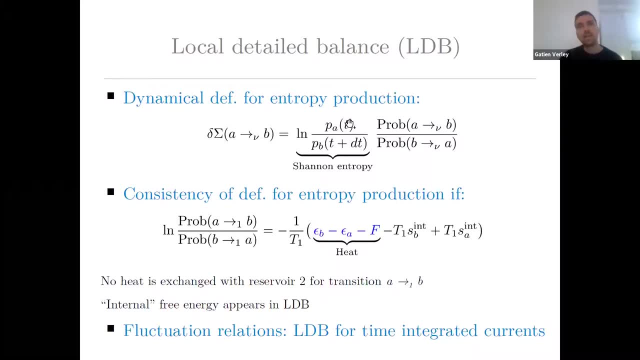 This was said by both previous speakers. This is what we expect, so that the entropy production is positive on average, And this is due to convexity inequalities. This is the positivity of the Kull-Black-Leibler divergence. So, from this statement and from the second law here, 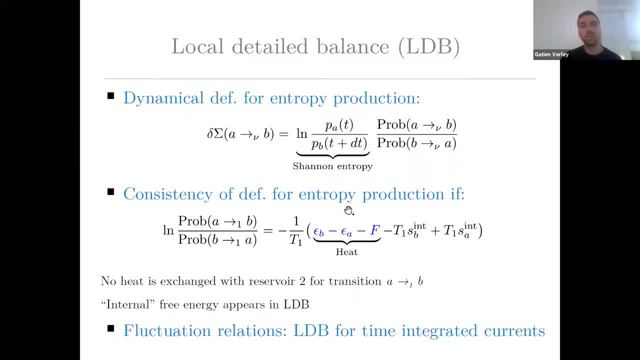 at the level of observable. you conclude that the log ratio of the probability in one direction and in the other direction, whatever your dynamic is, must be related to the heat and to the internal entropy. So actually we usually write energy, but due to these internal entropy states, 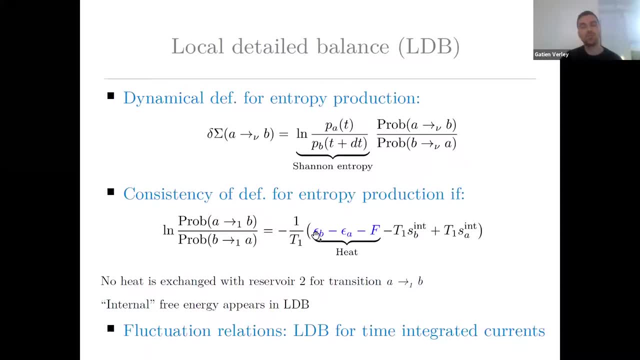 we should write that this is the log ratio of kind of free energy, which is based on energy and the internal entropy And the internal entropy of the state. So notice, as Jan Maria said, this is for the transition mediated by reservoir one. 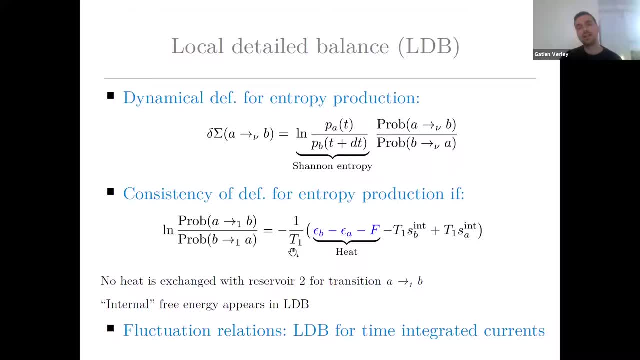 So the cold reservoir here, And then this is the temperature of this reservoir that is appearing in this local detailed balance. So that's it. This equation is stochastic thermodynamics. This is local detailed balance, is the fluctuation relation We know, for instance, 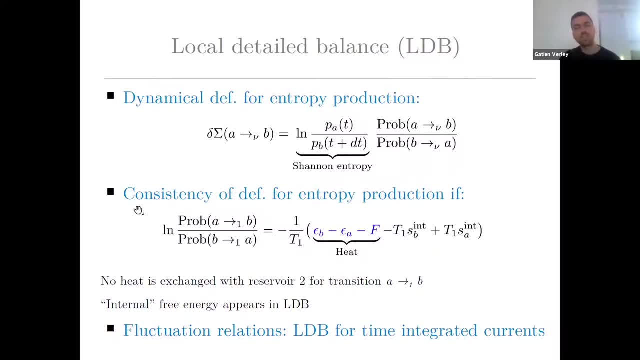 Sardzynski relation or other relations. When you just change the scale at which you look at your system, you look at macroscopic currents, then this equation is called the fluctuation relation And you have so many application of this framework. 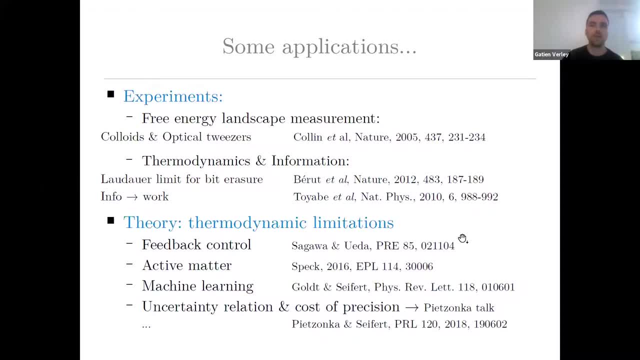 Once you have well defined your dynamics in terms of the thermodynamics, I mean when you have constrained it in terms of the physics. you have people that have looked at free energy landscape measurements, for instance optical swither and colloids stretching. 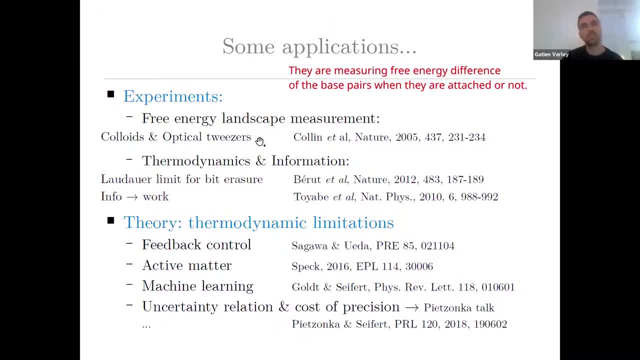 folding and unfolding DNA molecules and measuring ATP, free energy, ATP difference for the base pair when they are attached or not. You have people that have looked at the Landauer limit for bit erasure. So there is a cost in heat that is related to the fact of erasing a bit. 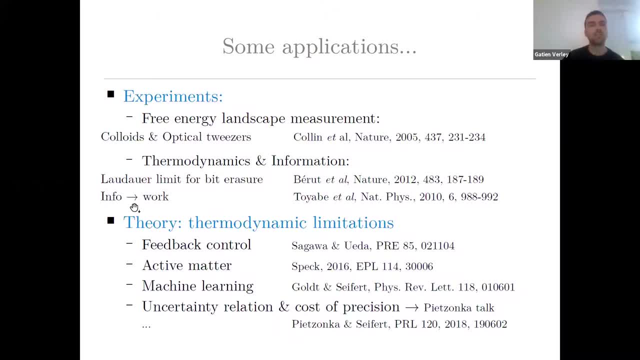 These are experimental investigations. You have people that have transformed information into work. on the theoretical side, People have studied the feedback control theory of thermodynamics, So they kind of had information inside the second law. You have people doing the stochastic thermodynamics of active matters. 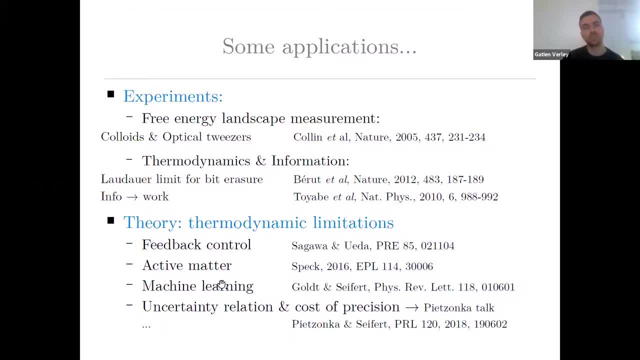 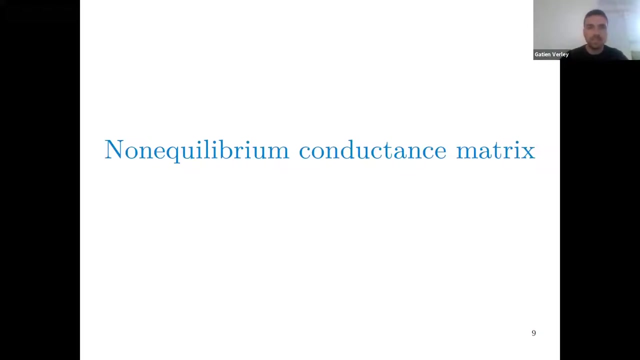 The one of machine learning, with the cost of learning and the level of known network of neurons. You have people, like in the talk of Patrick, who have looked at the cost of precision with these tools. I'd like to switch now with this basis that tells us that dynamics is 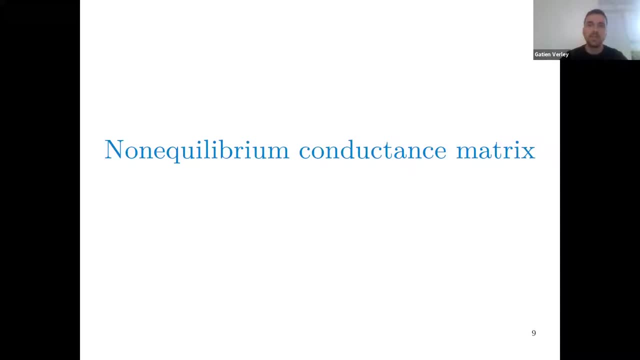 I mean of a system is constrained by the thermodynamics. Once you do that, you can go further to describe physical systems, And I'd like to describe machines, And to do this I have to discuss the physics of coupled fluxes. 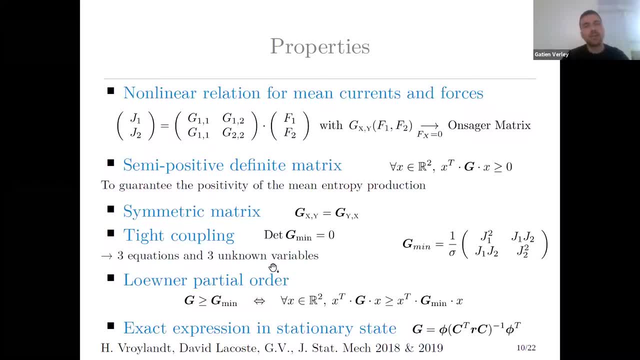 And a very interesting result we had was to generalize the force and flux relation through a conductance matrix that we call a non-Euclidean conductance matrix. that generalize Onsager response matrix. So Onsager response matrix is a constant here and it is related to the correlation. 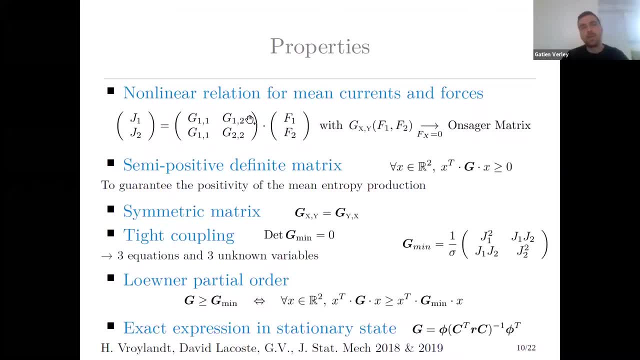 It is related to the covariance of the flux, But here this is not a constant anymore. This is a matrix that is a function of the force. in my system Here, if I want to do an engine, I need two forces and two fluxes. 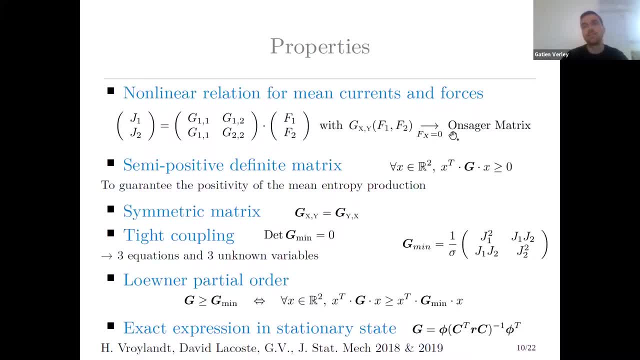 And obviously, when you go back to the vanishing force case, you recover the Onsager matrix. This non-linear conductance matrix is obtained through the description I've said once. you have well defined your rates in terms of the physical constraint. 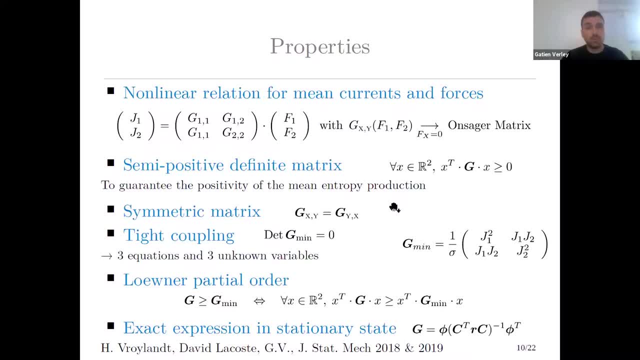 It is positive-definite, so that entropy production is positive. It is symmetric And this is very surprising. People know that the Onsager response matrix- I mean the response matrix when you look at response theory close to a non-equilibrium state. 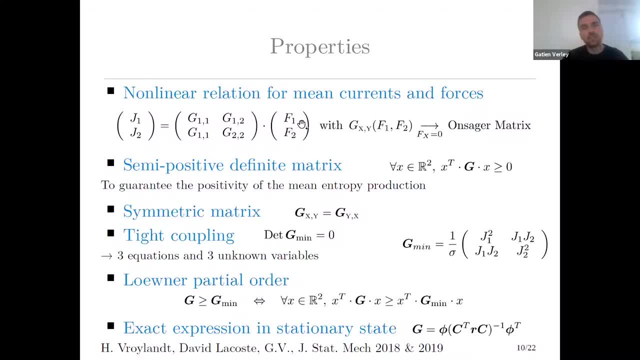 it is not symmetric, But this is due to the fact that this term includes order zero and one, and this one as well, So you have cross terms And then the final results. when you do this, perturbation theory is not symmetric anymore. 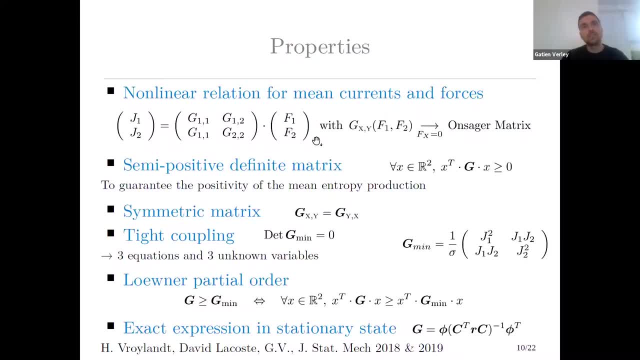 This object relating force and fluxes is much better than just the function, the current as a function of the forces. If you know the functional relation between the two, you have less information than if you know this matrix. You have one additional coefficient. 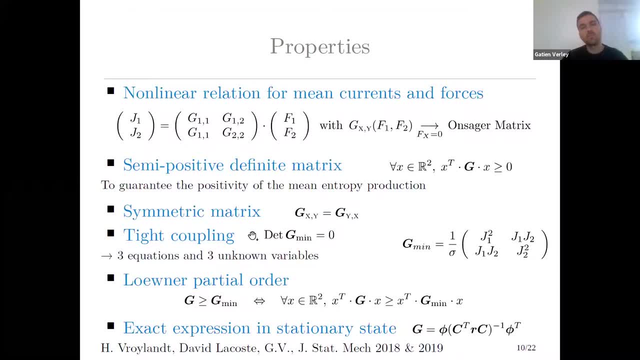 And this is at the core of the notion of tight coupling. The determinant of this matrix gives you a degree of coupling between your currents, And if the determinant goes to zero, you are in the tight coupling case and the matrix is directly related to the currents. 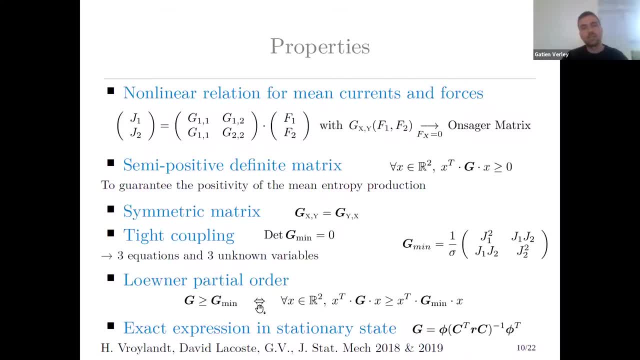 And you have inequalities on the matrix. Basically, such inequalities are just that the difference of the matrices is positively finite And you can add an inequality, for instance, for the covariance. So this is that: the fluctuation theorem, fluctuation, dissipation theorem. 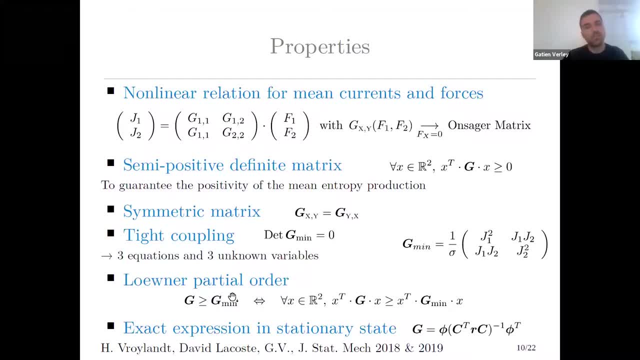 is now an inequality in the non-equilibrium case And this gives rise to all this stuff of thermodynamic uncertainty relations. I emphasize that this matrix has an expression that we can obtain from a physical matrix, which tells you how much is exchanged during various cycles on the graph. 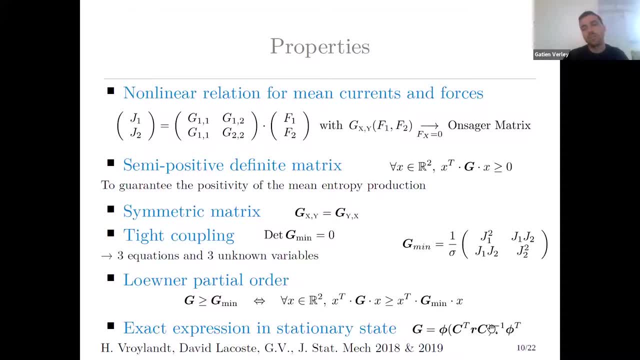 if you have discrete descriptions: the fundamental cycles, which is the basis of the cycles on the graph, and the local resistance, which is the ratio of the force divided by the stationary current along each edge on the graph. And okay, I don't go into detail. 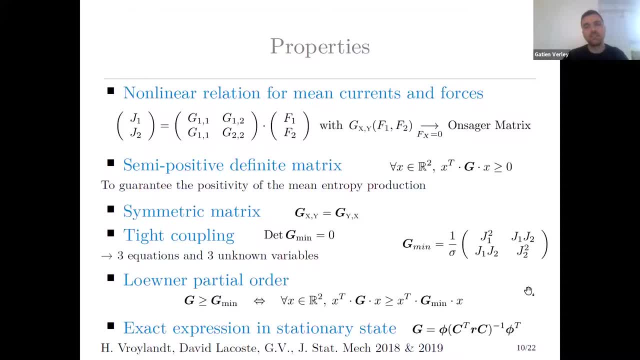 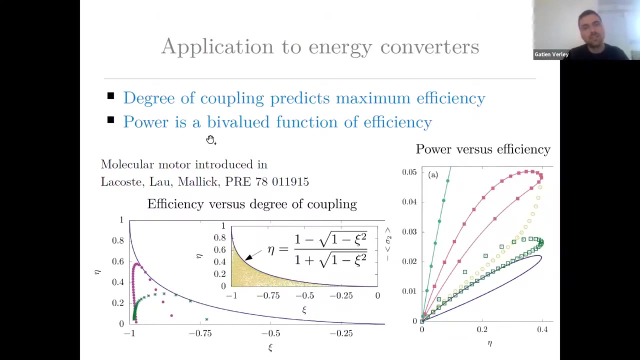 of this expression, but I emphasize the fact that once you have the dynamics and its stationary states, you know this matrix. So now what is important, as I said, is this notion of coupling between the fluxes And before the introduction of this matrix. 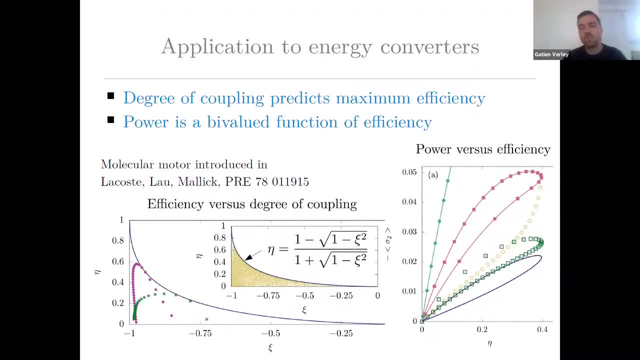 we just had the notion of: is the system in tight coupling and the two fluxes are intimately related or not? Here we can introduce the degree of coupling which is related to this determinant of the matrix, and it gives a bound, which is very simple, on the efficiency of an engine. 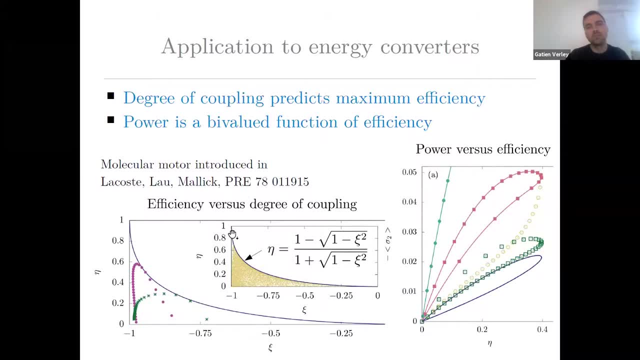 So we take, for instance here, a molecular model, We draw this bound in terms of this degree of coupling, which is no function of the forces, and we take random parameters for the model. and you see, it's working very well. 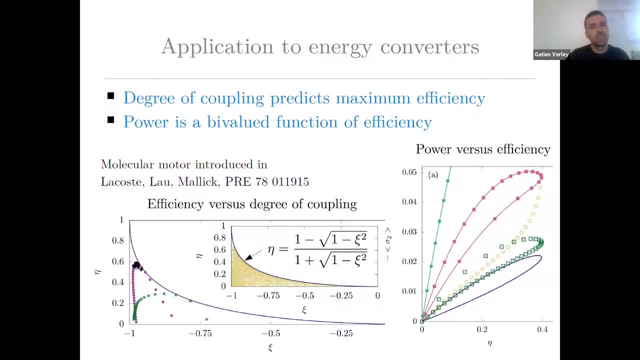 Or if you just take the forces changing for a given set of parameter, you see that you reach eventually this bound, but you never cross it And you recover in the tight coupling regime which is fully anti-coupled fluxes, the reversible efficiency. 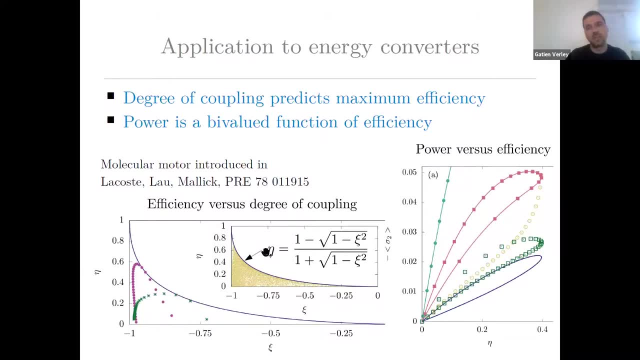 I mean the maximum efficiency, which is one because we are normalized. Another very nice result is that in the linear regime, you know that the power here is the power on this axis versus the efficiency which is the absolute function, which is a loop like this. 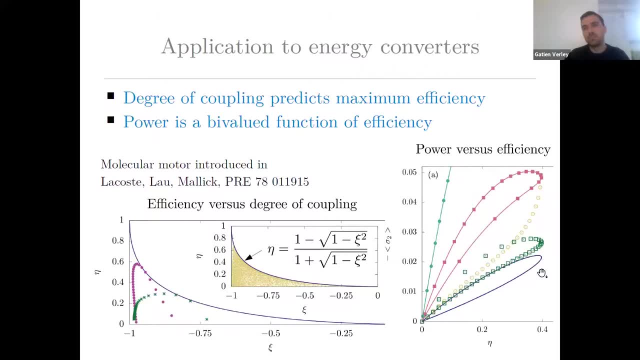 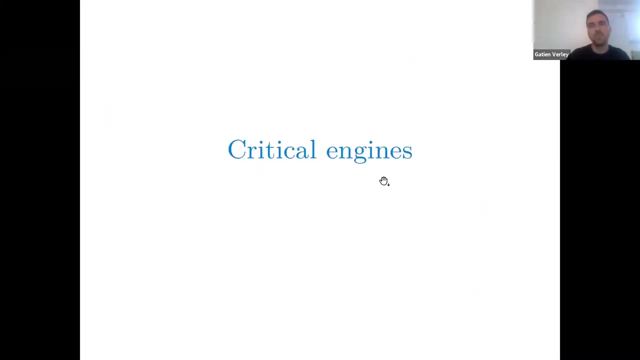 And you have the maximum power and the maximum efficiency there And we can show exactly for non-linear engines- far from equilibrium, that this shape is the same. You have loops for non-equilibrium- far from equilibrium- engines. So we have studied critical engines as well. 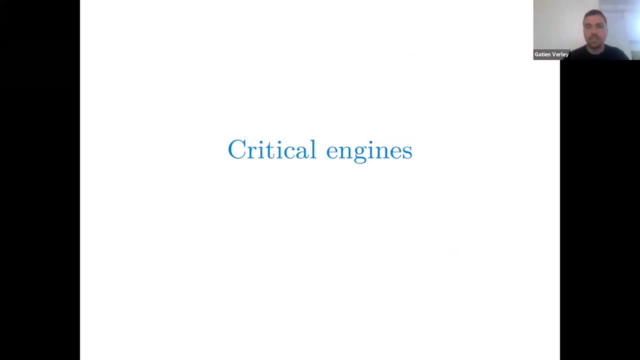 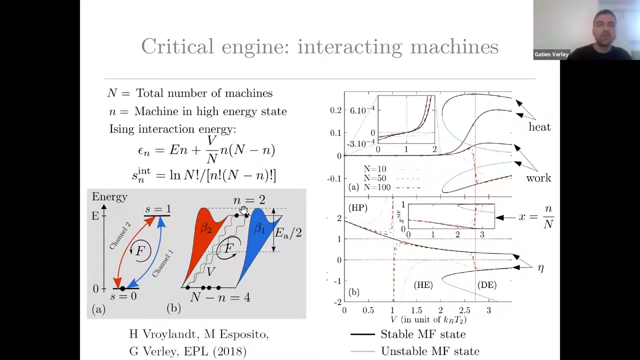 So engines that are undergoing a phase transition, And we needed this description, in terms of the degree of coupling, to understand what was going on in the critical engine. So this is the end of my talk. So this critical engine is made of individual machines that are unicyclics. 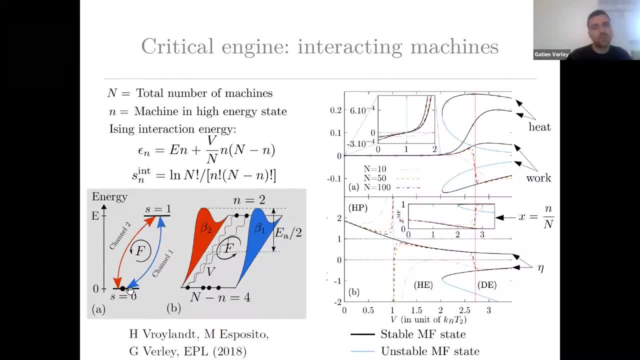 They have two states and two reservoir allows transition from these two states. This is an easing, like machines, but there is a non-conservative force that allows to collect work And we had an interaction energy to this machine. We take many of them. 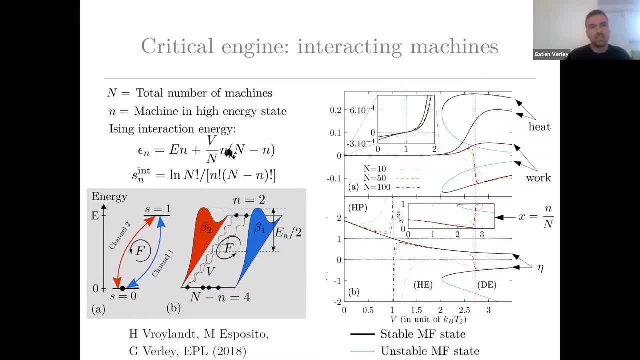 actually N capital N of them, And the interaction energy is the easing one. So the machine tends to go into the same state. But there is this internal energy state that is due to the combinatoric, the many way of putting the machine. 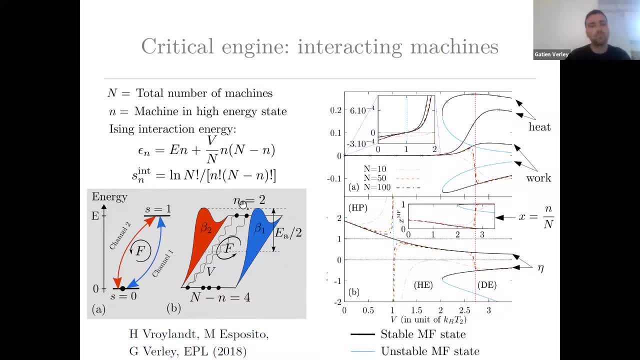 in the value states. that tends to split the machine between the two states. So this competition is leading to a phase transition, Which is very famous, And you have a bifurcation diagram for the density of machine, for instance in the upper state. 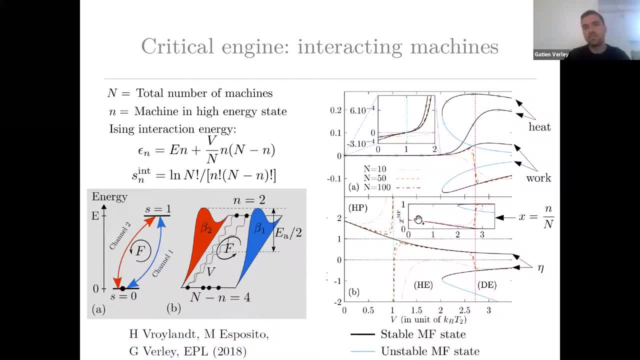 And when you increase the interaction V energy, you see that your density, I mean you have two states, mean field states, that three that appear to stable, one unstable, And you eventually have a transition from one to the other. The dash curves are for finite size machines. 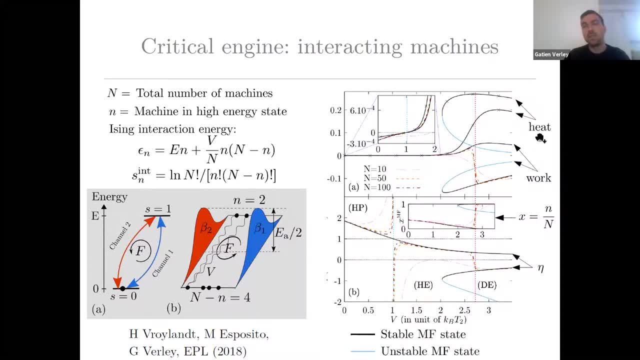 Finite number of machines And since the heat and work fluxes are function of this density, you can look at the mean field, the heat and work fluxes that also undergo bifurcation diagram with a transition. And there is work here. Here is work that is produced. 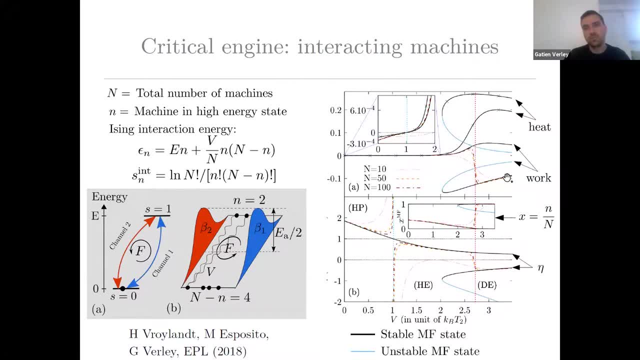 And then the machine change of state due to the transition and go to a third engine And if you have the fluxes, you can also look at the efficiency of the engine. And this is this plot here. Here is the efficiency I'm showing. 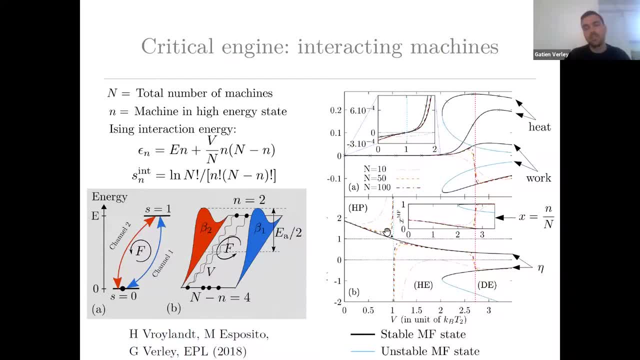 Here in this sector the efficiency is actually not the right one, because in this sector the machine is a heat pump, So the good efficiency is one over the efficiency that is shown here. So good thing, the mean field efficiency is lower than the reversible one. 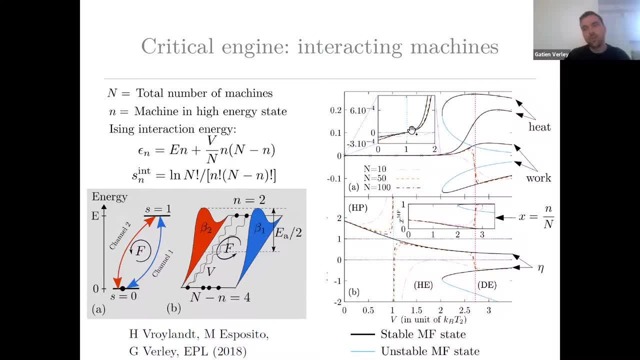 But when the current change of sign- so this is a zoom here and the change of sign is close to one- then the machine change of working regime and go to the heat engine regime and will eventually, if you still increase the interaction, it will reach the dead engine regime. 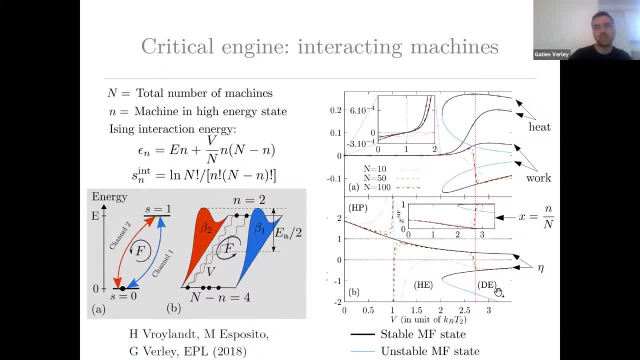 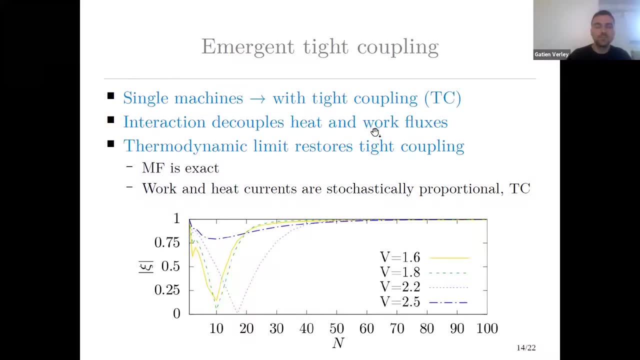 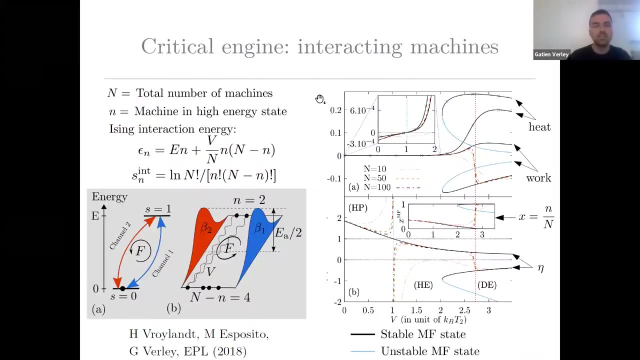 So we are able to study in great detail on this toy model, the mean field case, but we can also study the fluctuations. But first we had to face something peculiar with this machine, which is the emergence of tight coupling. So the single machine is unicyclic. 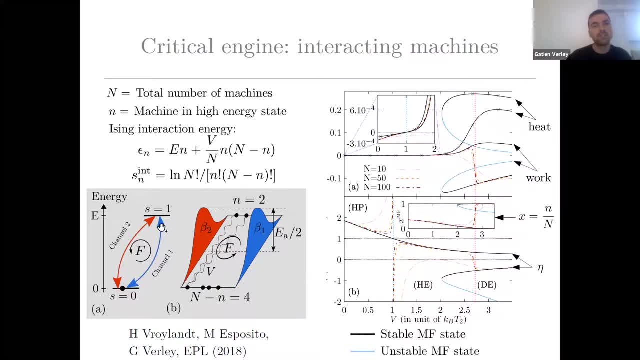 which means that for each heat flux that is given by the alt reservoir, you have a given amount of work which is given, And this is why the flux for this machine are tight coupled. If you introduce interactions, you decouple these fluxes. 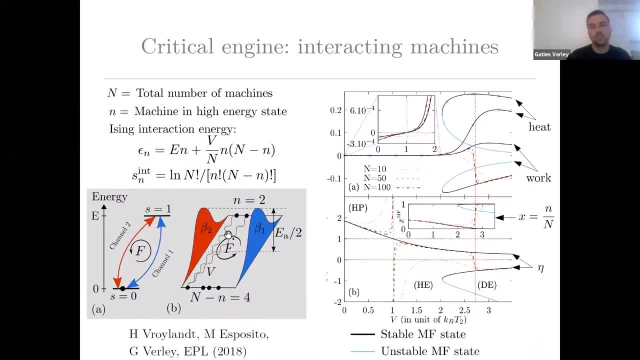 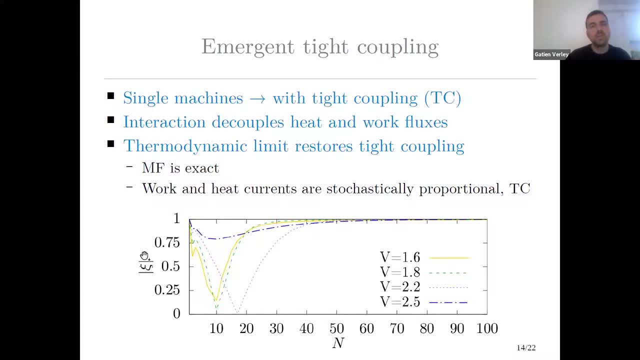 because you have many cycles. that can be done by the various machines. But if you go to the thermodynamic limit you restore the tight coupling And this is possible to see using this degree of coupling parameter, which was defined in my previous part as something related. 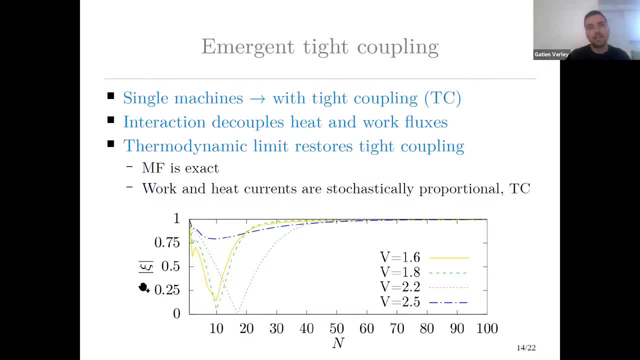 to the determinant of the matrix, And here we take its absolute value. If the degree of coupling is one- here I mean its absolute value is one- it is tight coupling. So when the number of machine n is one, we have this tight coupling. 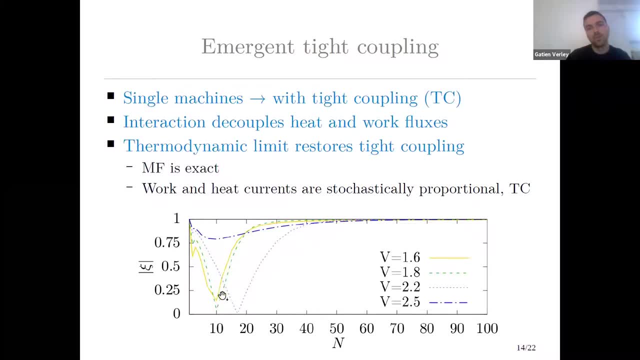 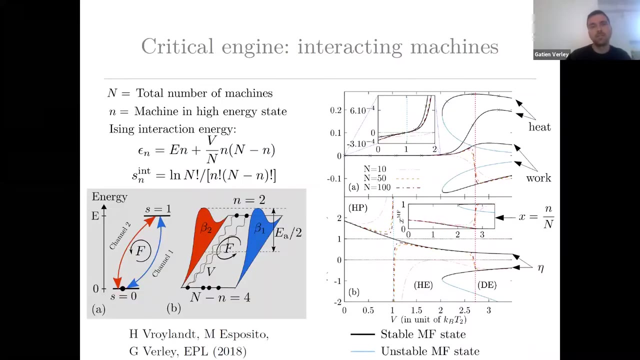 We increase the number of machines, the degree of coupling goes down And then, due to the macroscopic limit, it goes back to minus one, which is here one, because it's absolute value, And this can be understood, because the machine, in its Milfin state, 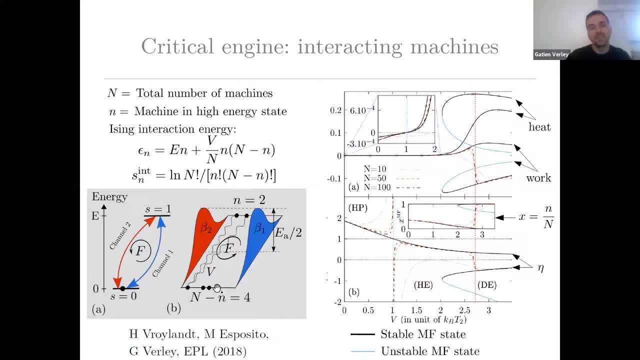 basically all remain in the same state And when you have a transition, there is just one machine going to the other state and coming back. So there is effectively just one cycle which is made by the machine. So that's why it comes back. 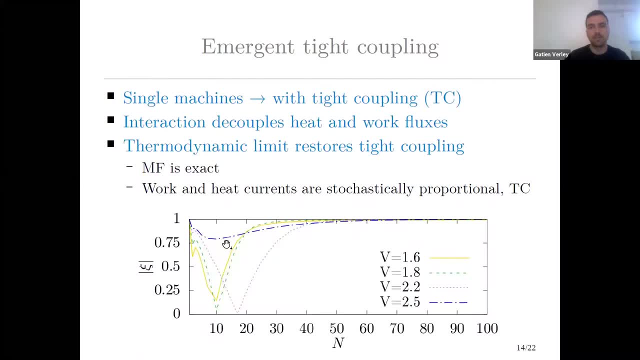 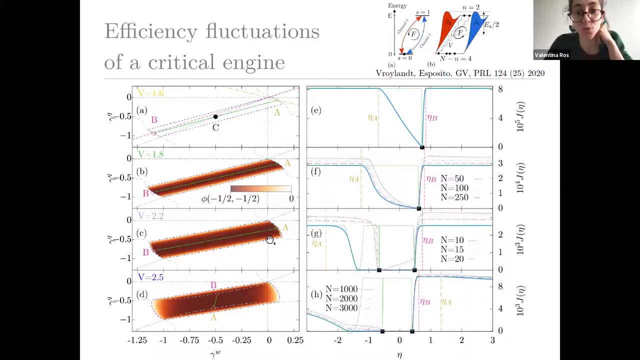 to tight coupling machine in the macroscopic limit. Sorry, More or less one or two minutes. Yeah, I'm done almost. So if I study the efficiency fluctuation of this machine, I can look at the probability of having a given efficiency here. 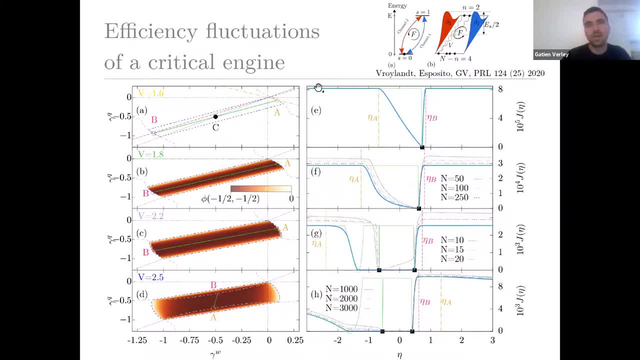 So this was a very involved work to have analytical results for these machines And we can get the cumulon generating function of the work and heat. So this is the Laplace. I mean the conjugated parameters to the work and heat. 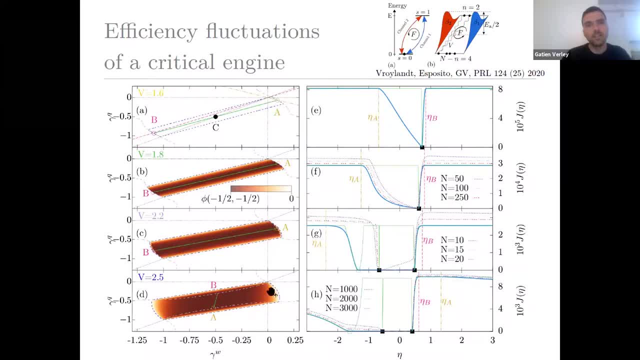 So the derivative close to zero here gives you the mean values. But here we have all the cumulon generating function in the whole space And if you from this you can actually contract to get the efficiency fluctuations. So I don't give you the details. 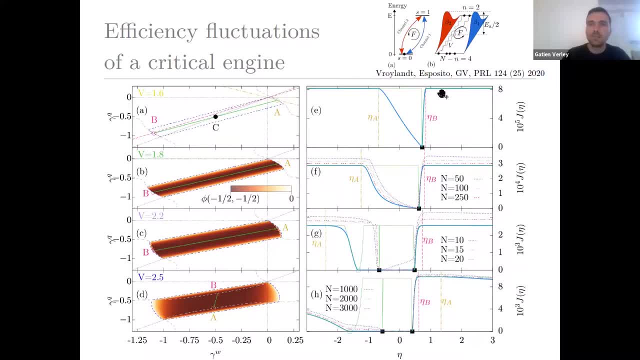 I just give you the physics. We had the results saying that the reversible efficiency is the least likely, which corresponds here to the maximum. because we are studying large deviation function, which are kind of potentials here for the efficiency. I say kind of, because they are not potentials. 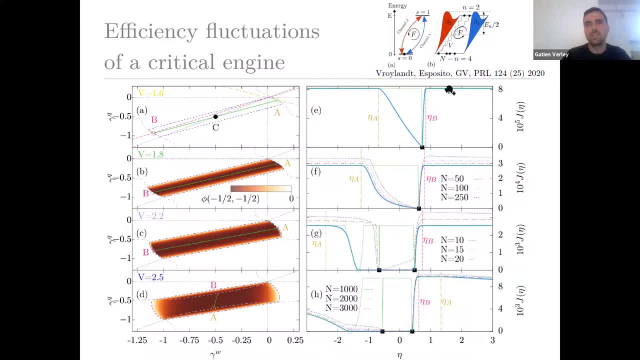 But here we see that there is a degenerative function of the maximum and also after the transition which goes here. the transition is there from V2, 1.8 to 2.2. You have coexistence between different value of the. 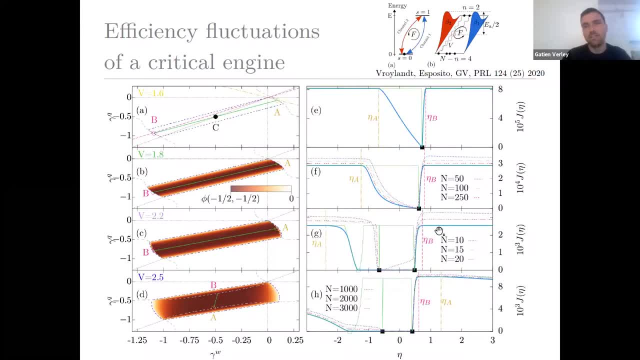 most likely efficiency and you have degeneracy of the least likely efficiency as well, And this is due to the tight coupling which is emerging and which, in the cumulon generating function, is generating plots are due to these lines that appear. Actually, there is only one line. 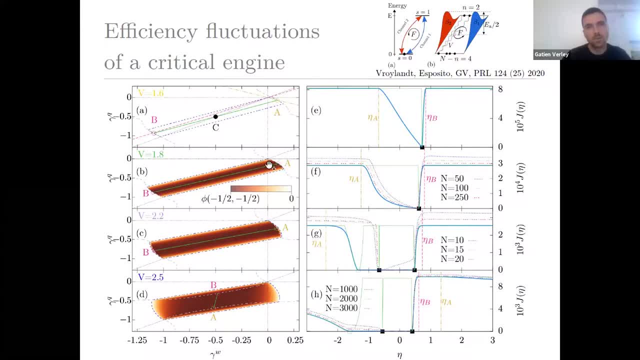 which is the bottom of the. Here is a color plot and you see the darker is here. and this is the minimum of the function, the cumulon function. So this is the least likely, which is at the minimum and the most likely. 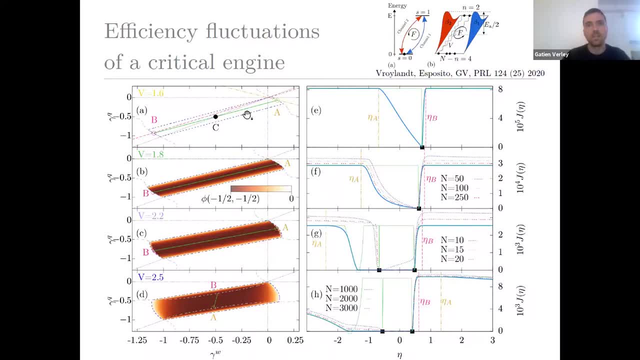 which is at the maximum here around the origin. I'm not showing what happens outside the boundary because it does not matter for the efficiency of the least likely fluctuation curves And we also did the finite size computation with the convergence to the large deviation function. 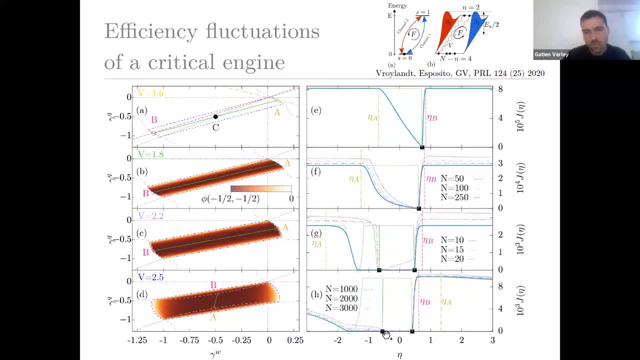 And I just comment that it converge much faster to the stable case than to the unstable plateau here. And okay, there is ergodicity breaking thing. So you have the ergodic case in blue and the non-ergodic case in green, And there is lots of physics you can do. 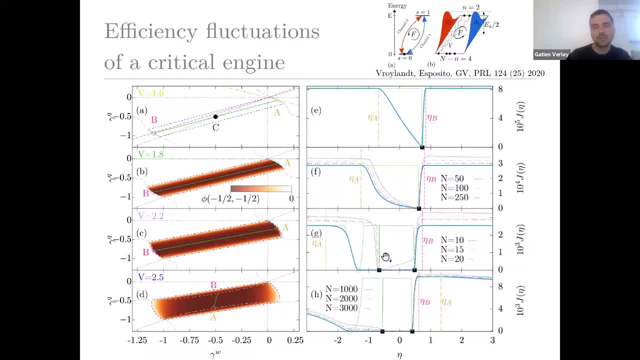 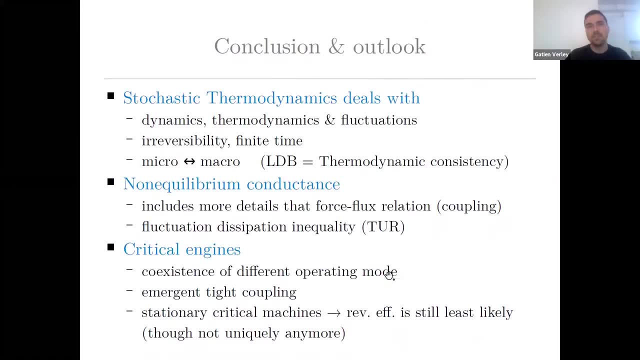 here, considering that you have mixture of states where the machine is actually working as an engine and where it is actually a dead engine. Let me summarize what I just said. So I have quickly introduced stochastic thermodynamics and I have emphasized that at core of it is local detail balance. 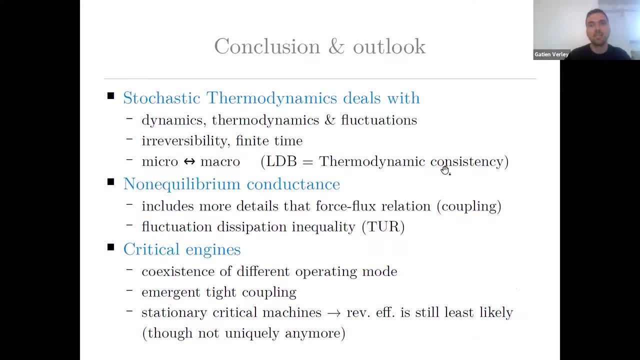 which is a dynamical constraint answering thermodynamic consistency, and which is a connection between microscopic and macroscopic dynamics. I have told you that, given that I'm able to describe small systems that are more often out of equilibrium, far from equilibrium, I can study the nonlinear physics. 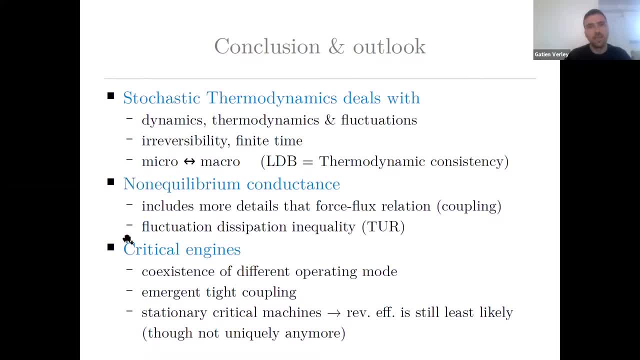 that goes with it, which generalize the work of Onsager, And we went further and looked at critical engines and their fluctuations. So here I studied efficiency fluctuations a lot and basically we were motivated into checking if the reversal efficiency is still the least likely. 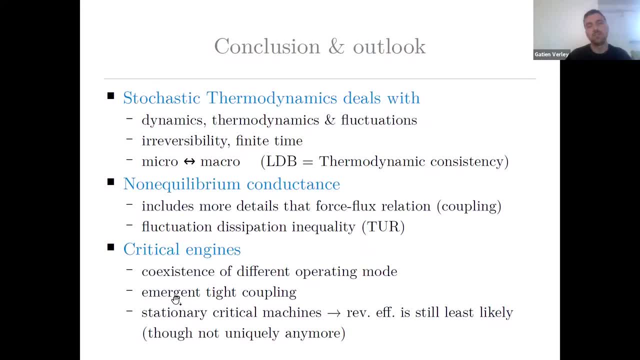 and it is true even though you have non-convexity of the large deviation function and you have ergodicity breaking. But the only thing that is not true anymore is that you can have several efficiencies that are the least likely in the large time limit. 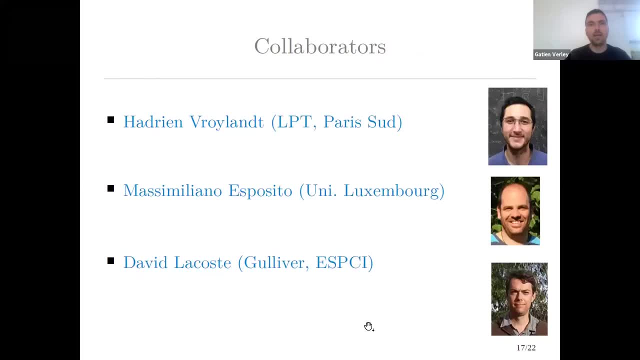 and that's it. I thank the collaborator with whom I did this work: Adrien Voilant, who was my PhD student and who did a lot of the work I presented, Massimiliano Esposito and David Lacoste, who has worked with us. 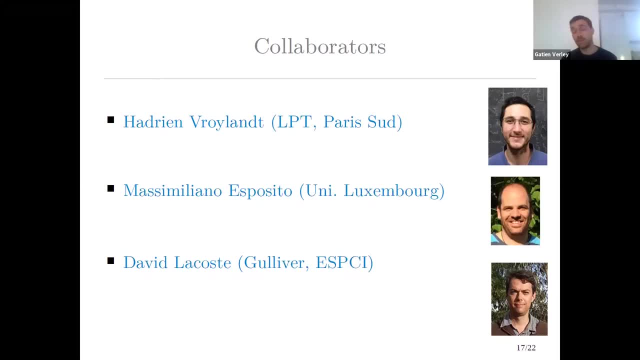 And I end by thanking the organizer for the invitation and you for your questions. Thanks a lot, Gathian, for the talk. So is there anybody? We have time? Yes, There is Isaac. Please go on. Yeah, I had a question. 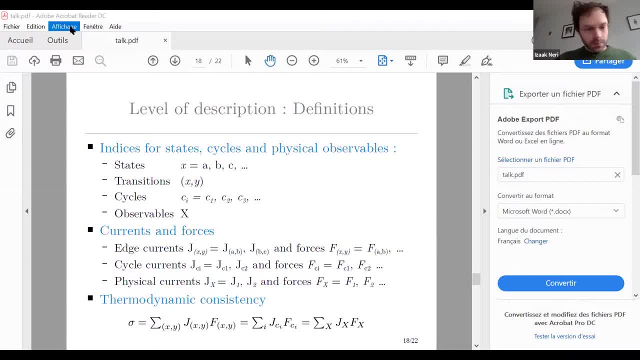 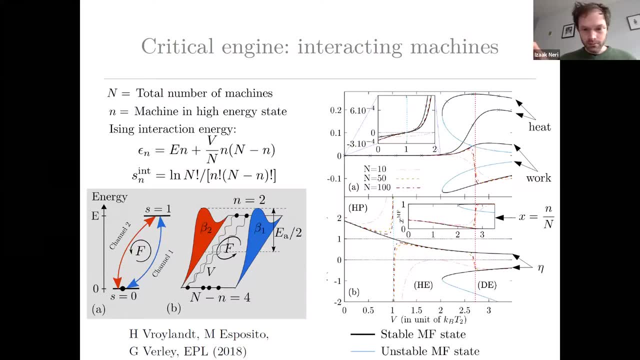 about those critical engines. I think Patrick Pechonka mentioned yesterday that you can have Carnot efficiency at high power if there's a large number of fluctuations in the power. Is it something you can observe as well in those interacting machines You asked? 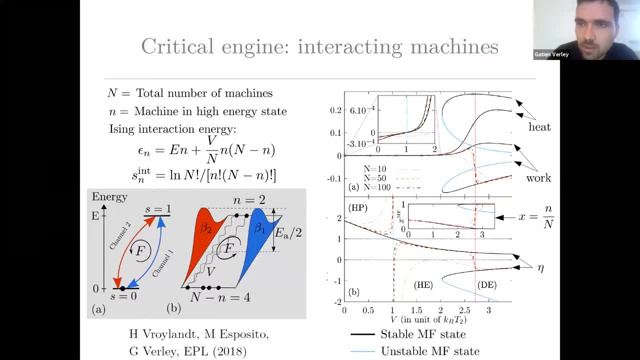 I mean precisely if you can have finite power and reversible efficiency. Yes, exactly. So you have people arguing that, due to scaling in system with phase transition, you could have that. So this I would agree, but it is very important. I mean, I don't believe. 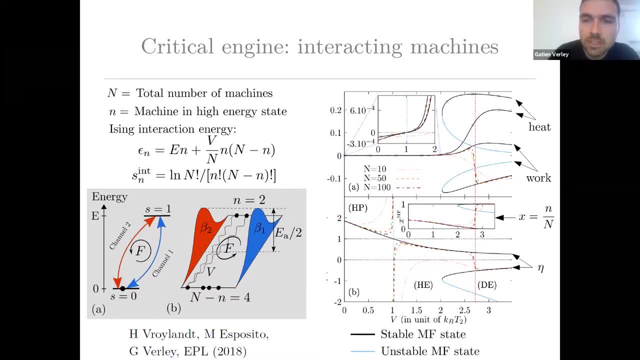 that you can have finite power and reversible efficiency. For me it is impossible. I am the one who agree in this direction, because usually it goes into the case where you are dealing with these tight coupling engines, which is already a very mathematical limit. 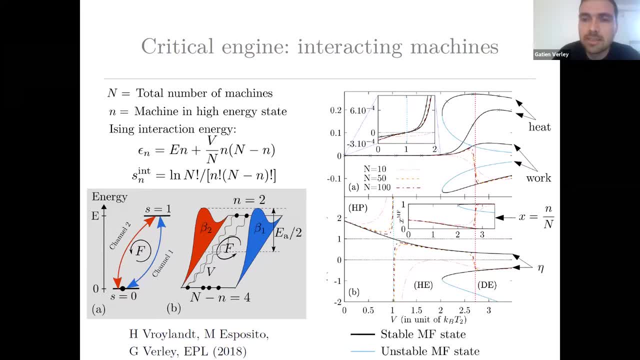 And the other things which is required to have finite power at a reversible efficiency is infinite forces, which is also a very mathematical thing. So, in the end, the only way I could imagine that something is happening- but I would say I don't believe it-